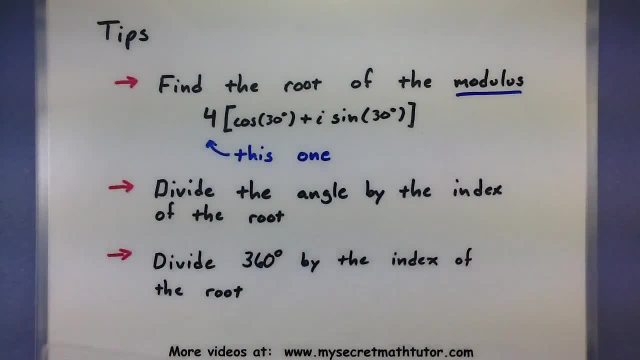 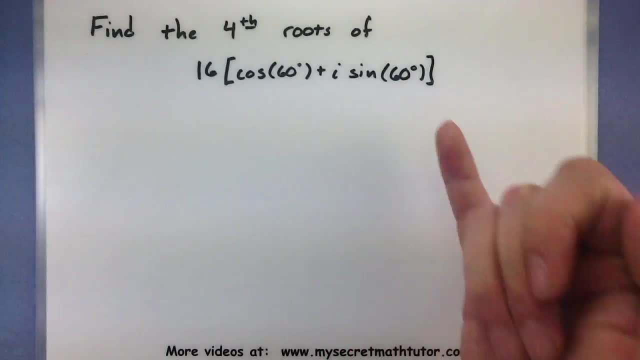 need. Let's give it a try with an example problem. I want to find the fourth roots of 16 cosine of 60 degrees plus i sine of 60 degrees. So let's run down my little steps here, Do it one at a time. 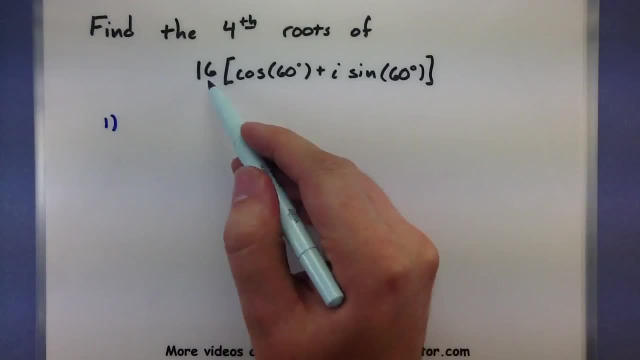 So the very first thing you want to do is: let's find the fourth root of the modulus, So fourth root of 16.. Well, that's not too bad. The answer to that is simply 2.. Now, what else do we need? I want to take the angle, whatever it is, and divide it by the index. 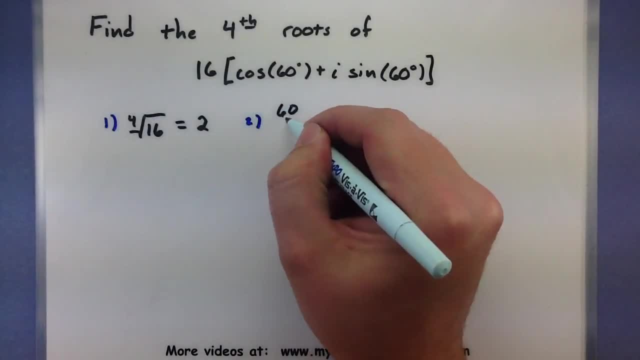 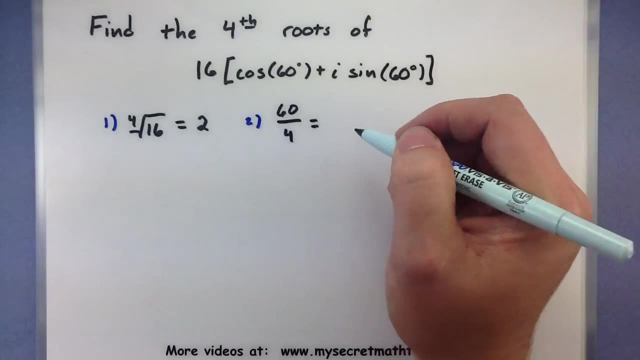 of the root. So our angle right now is 60. And the index of my root- since I'm finding the fourth root- is 4.. So we'll take 60 divided by 4.. Well, that's the same as 30 over 2, or 15 degrees. 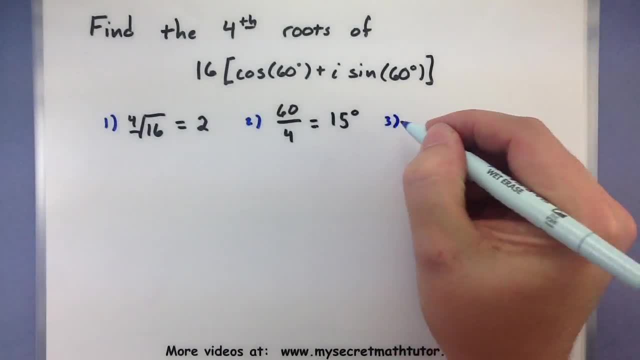 One more thing we need to find is we need to take the entire 360 degrees for our circle and divide it by the index of the root, So 360 divided by 4.. So if you think of a circle chopped up into four, you'll get 90 degrees. Now that you have each bit of information, 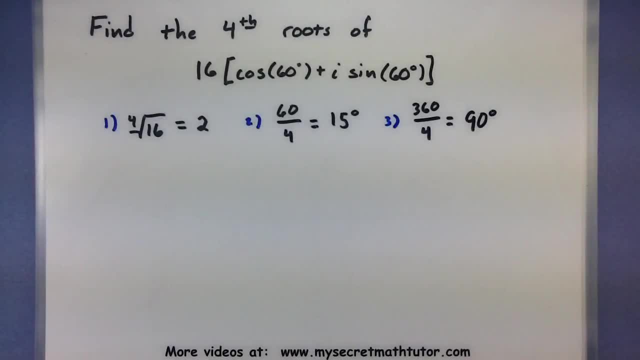 now watch how we put these together to build all of our roots. All right, So what is the first of our roots? We'll have four of them in total. Well, the first one. we'll use the fourth root of the modulus cosine of this angle: 15 degrees. 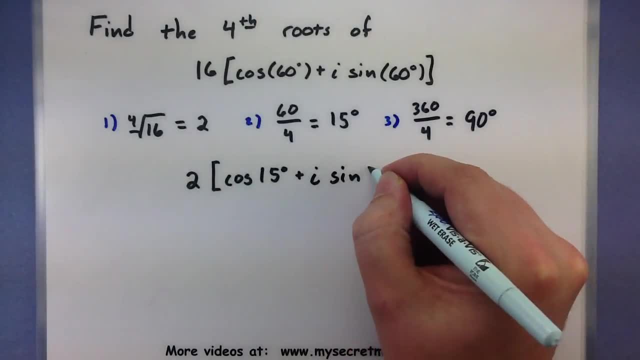 plus i sine of 15 degrees. Okay, And there's our first one. Now, since we're doing the fourth roots, we should have four in total And using just this and this, you can get the first one. The reason why we found 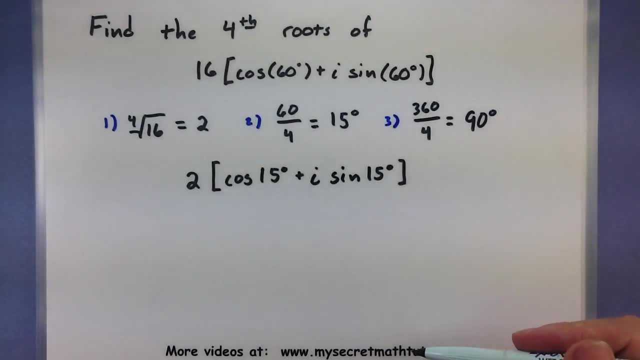 this third bit of information is that will tell us exactly how to get the rest. We simply add 90 degrees for every single one after that. So what do we do about the two? It actually stays the same for all the rest. So 2,, 2,, 2.. And now we're going to go through and add: 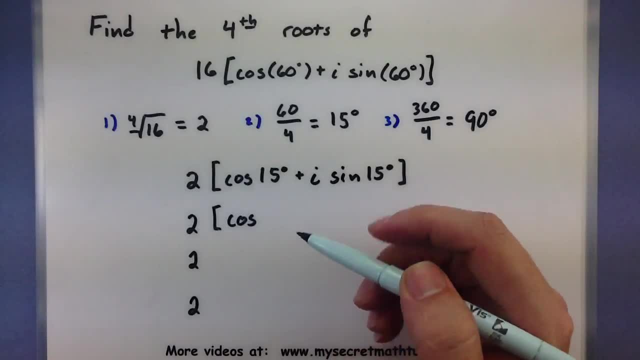 90 degrees. for every other one, 15 degrees plus 90 degrees. that'd be 105 degrees. 105 degrees, All right, Add another 90 degrees to that one. Now we're at 195.. All right, Keep going. Let's add another 90. 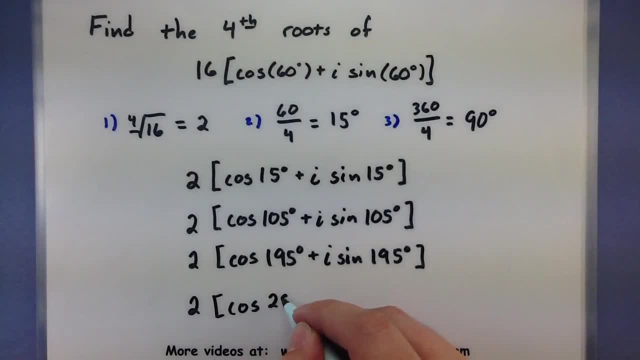 degrees to 195.. So we have 295.. All right, 285 degrees. Now, if you accidentally forgot to stop, even after you got four, what you would end up doing is you'd get an angle that is coterminal with your 15, so it would essentially start. 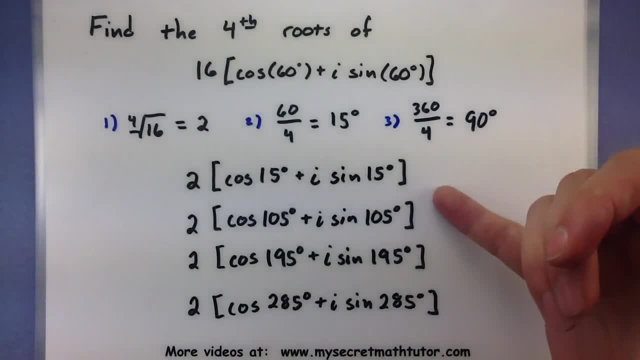 repeating back over. But now that we have all four of our fourth roots, we can say that this one is done. So remember, find those three bits of information, like the index of the modulus, Divide your angle by the index of the root and divide 360 by the index of the root. and 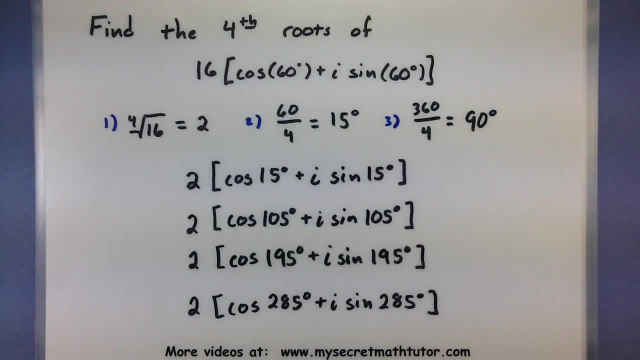 then put it together carefully to build all of your roots. If you'd like to see some more videos, please visit MySecretMathTutorcom. 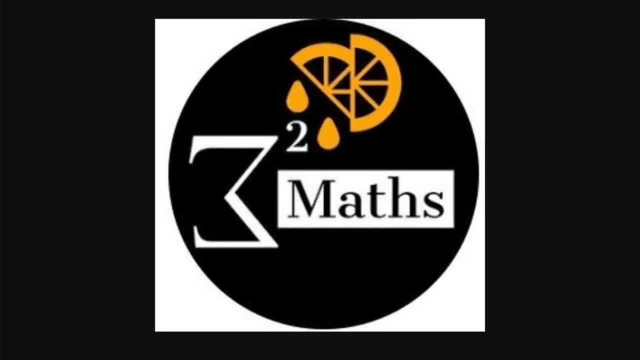 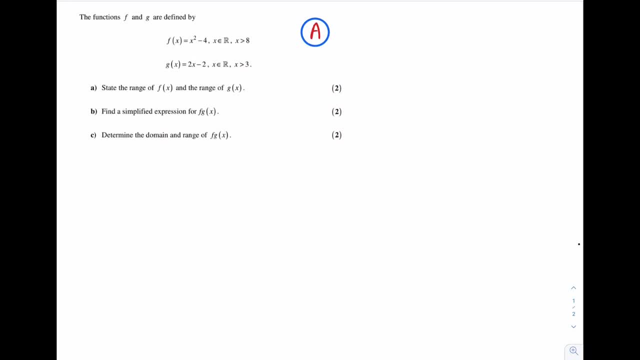 Here is an A grade question on functions, domain and range. The functions f and g are defined by: f of x equal x squared minus 4,. x is an element of the real number set. x is greater than 8.. g of x is equal to 2x minus 2, x is an element of the real number set. 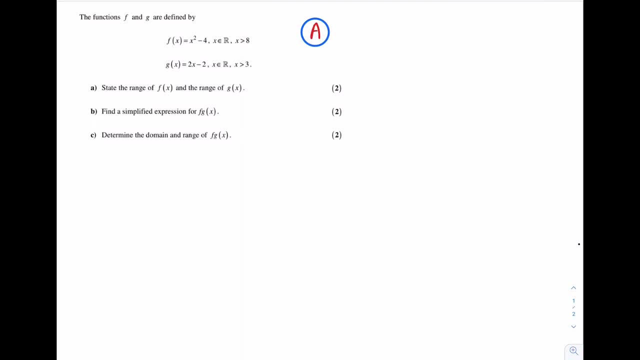 x is greater than 3. Part: state the range of f of x and the range of g of x. Part. find a simplified expression for f of g of x. Part. determine the domain and range of f of g of x. This question is worth 6 marks. Pause the video. have a. 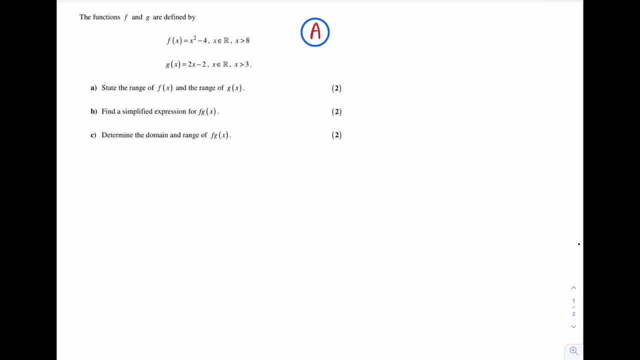 go at the question and play the video. Let's have a look at part To find the range of f of x and the range of g of x. it is particularly useful to sketch the graph of f of x and the graph of g of x.